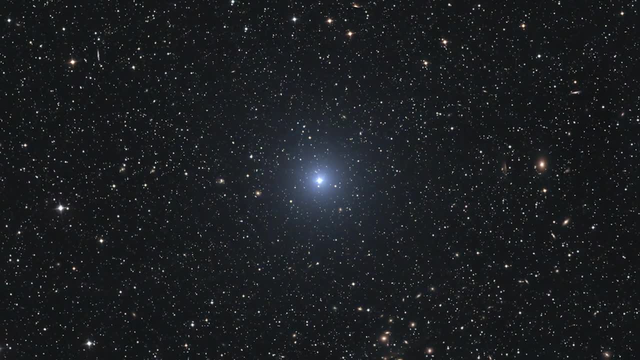 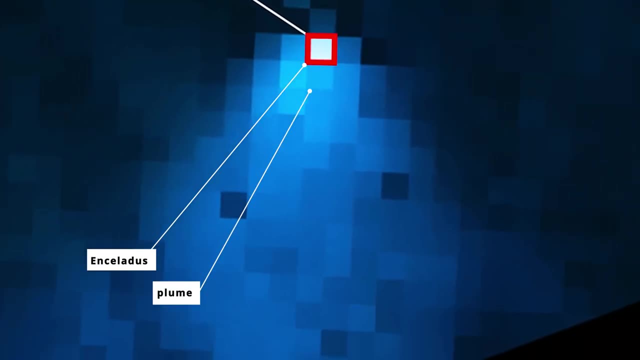 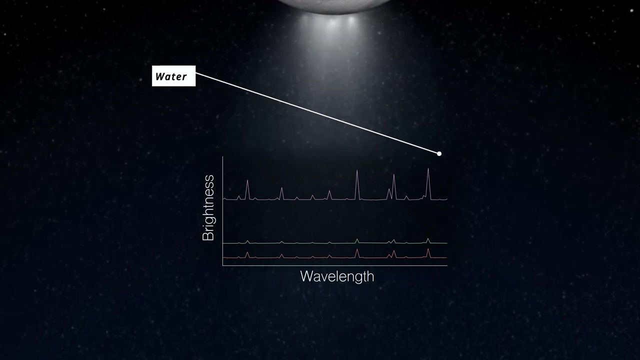 different wavelengths of light. Many objects or phenomenon are simply too far away to directly image. A lot of data comes from pixel-sized point sources, and those points provide astrophysicists with a powerful window into what makes up the universe, Even now. 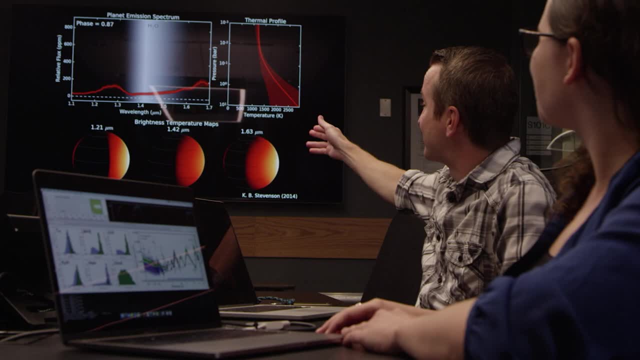 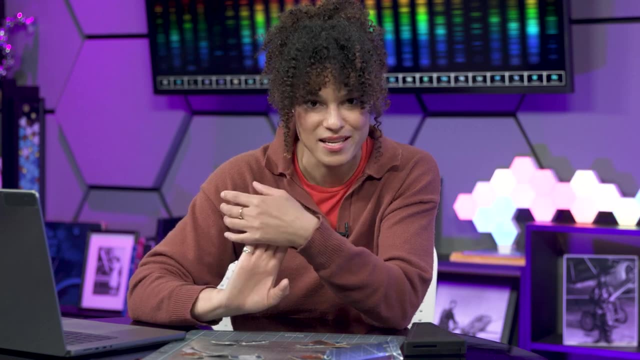 most of what scientists learn about the cosmos comes from studying light. Astronomers can work out distances, speeds, sizes, temperatures and the composition of elements, because matter behaves in a way that makes it possible for us to understand what's going on in the universe. 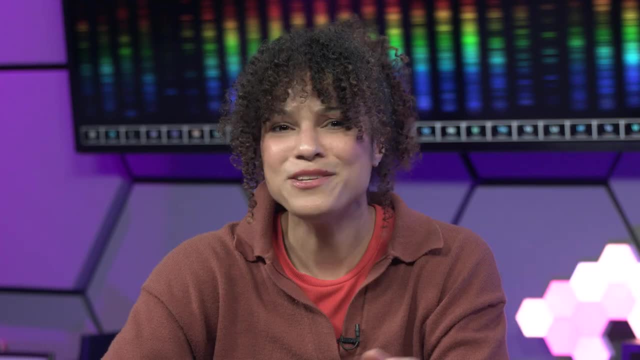 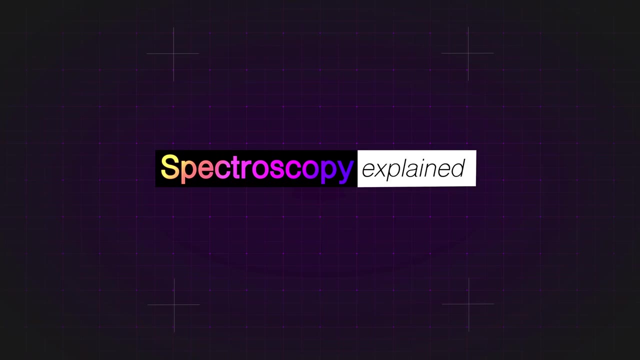 Because matter behaves in a way that makes it possible for us to understand what's going on in the universe. They do this in predictable and consistent ways. They do this by literally prying these photons apart. This is spectroscopy. Explained Spectroscopy is a study of how matter. 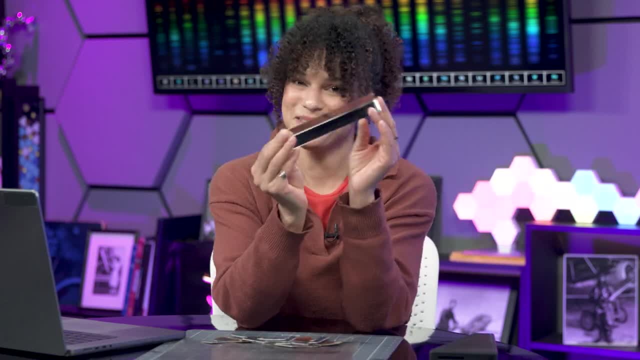 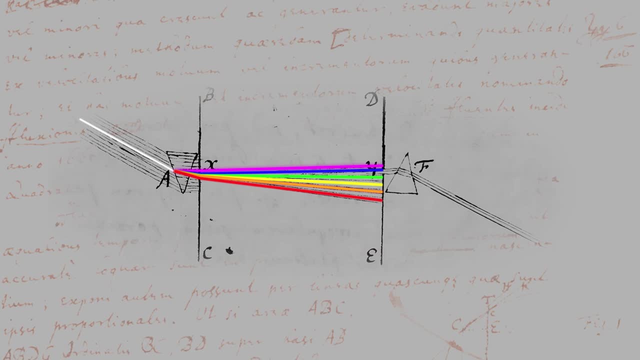 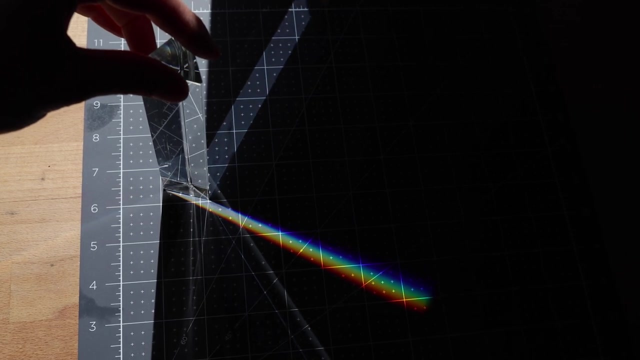 interacts with light, And it all began with a prism like this one. Light entering one side of the prism bends or refracts as it passes through the triangle shape and exits out the other side. All of the wavelengths enter together, but they exit as a rainbow-like spread of colors. 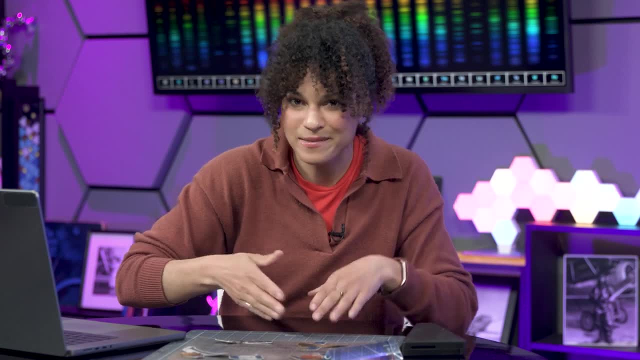 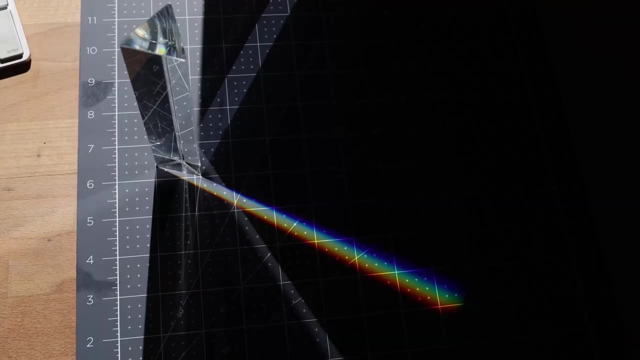 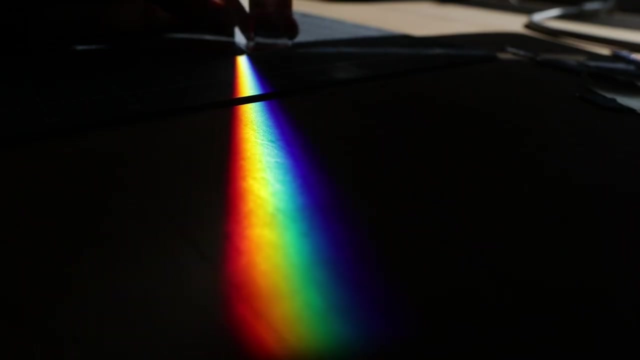 What's happening is that the shorter, more energetic wavelengths like blue and violet bend a little more than the longer lower-energy light like red and orange. Because they bend at slightly different angles, the wavelengths separate, fanning out into a band of colors. NASA has been working on a new study that will help us understand what's going on in the universe. NASA has been working on a new study that will help us understand what's going on in the universe. NASA has a whole fleet of telescopes that can split and study a wide range of light. 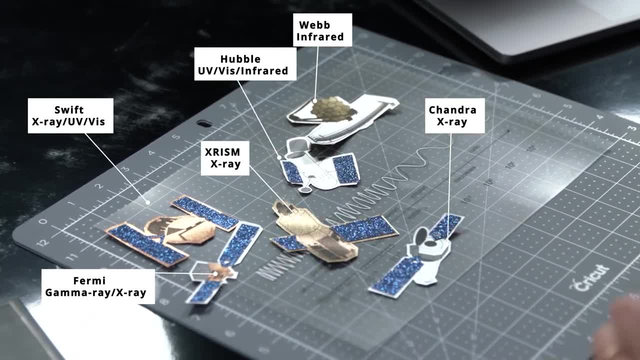 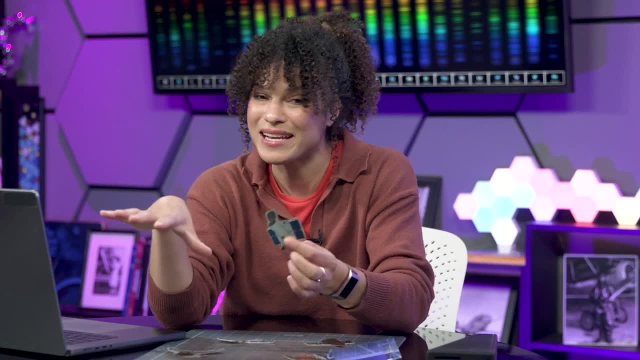 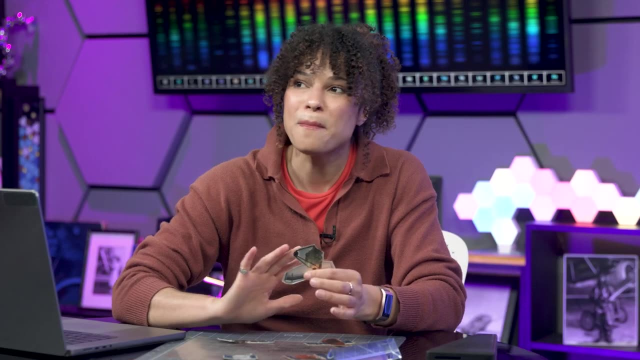 on the electromagnetic spectrum, not just the light that our eyes can detect- So Hubble can detect through the visible spectrum- but also a bit into the infrared and the ultraviolet. Webb is just infrared and can look at the light that is emitted from. 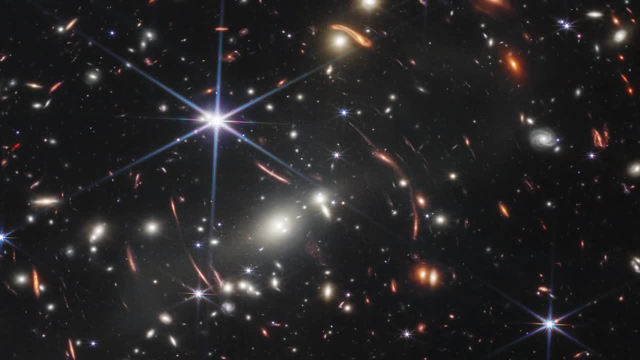 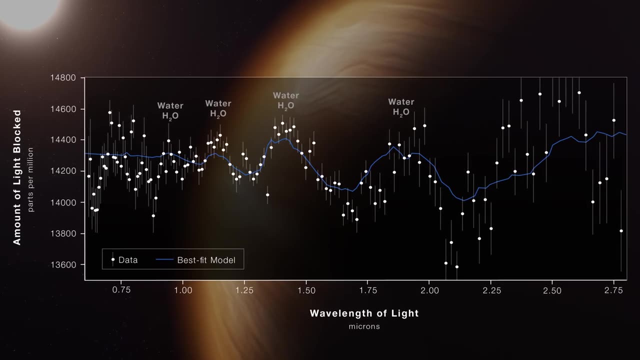 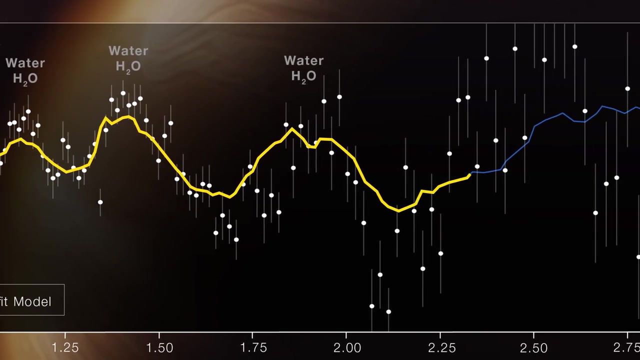 billions of years ago, And, of course, the images from Webb are really spectacular. But this, This is what flutters the hearts of scientists. This spectrum shows a light that penetrated the atmosphere of a planet called WASP-96b. The light being measured comes from the planet's host star, some of which skims through the 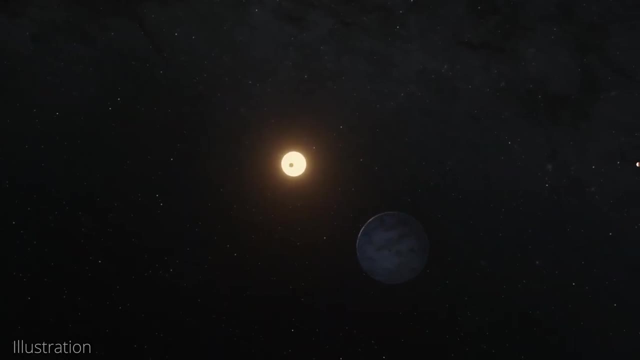 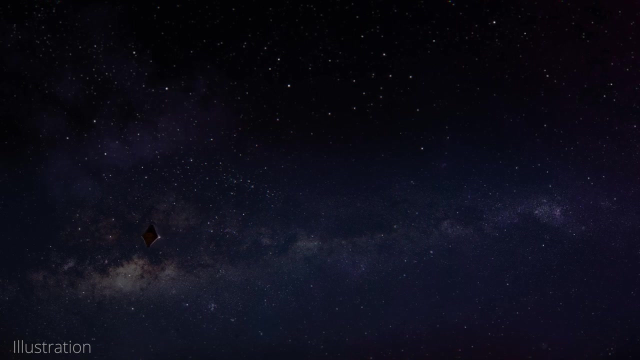 atmosphere. Humans are a long way from directly imaging exoplanets, so telescopes like Webb will use spectroscopy to find those chemicals that could support life in their atmospheres, Which is why Webb's first spectra is so amazing. You're actually seeing bumps and wiggles that indicate the presence of water vapor in the 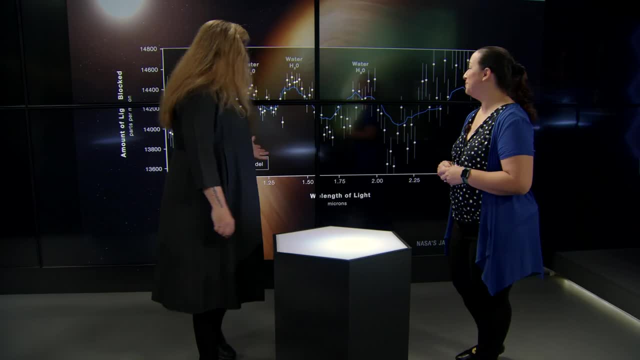 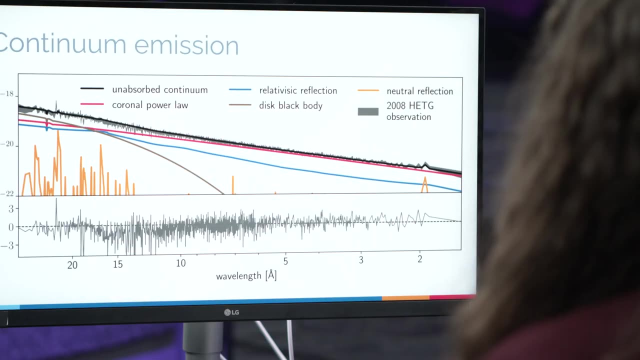 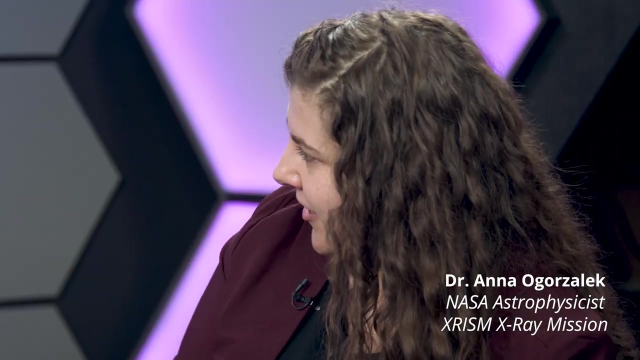 atmosphere of this exoplanet- Incredible. But it's one thing to identify single elements or simple molecules, but deciphering whole foreign bodies like Dr Owa Jatowek, How do you know? Oh my god, it took us a very long time to figure this out. 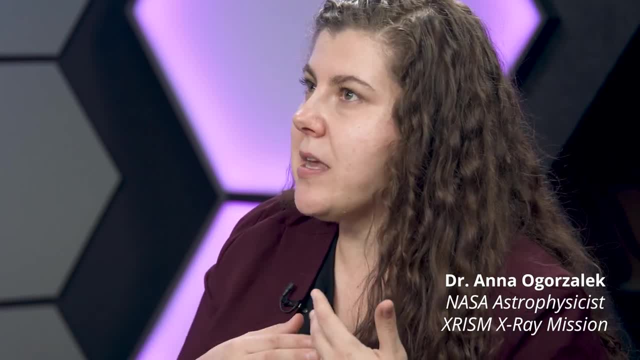 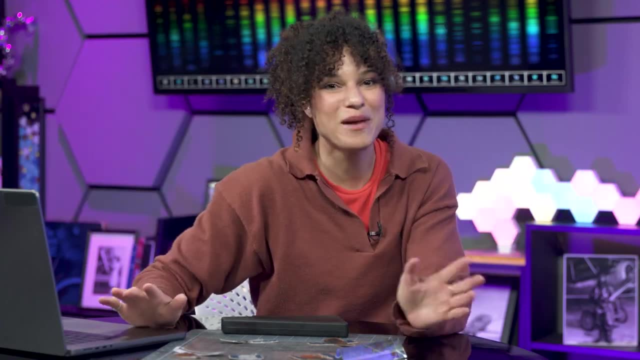 It really took us many, many decades, and it took us many, many fantastic new instruments. If all of our astrophysical objects, or anything that we're looking at, were made up of one element, this would just be so easy. But we don't. 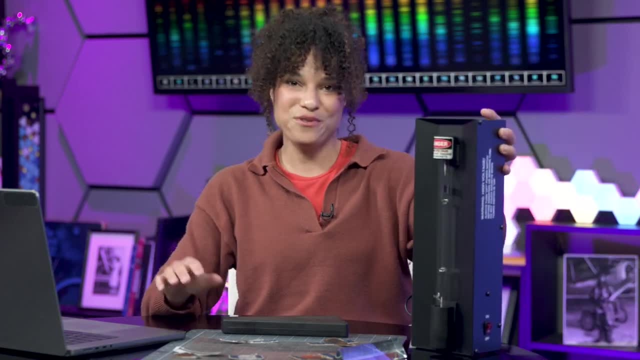 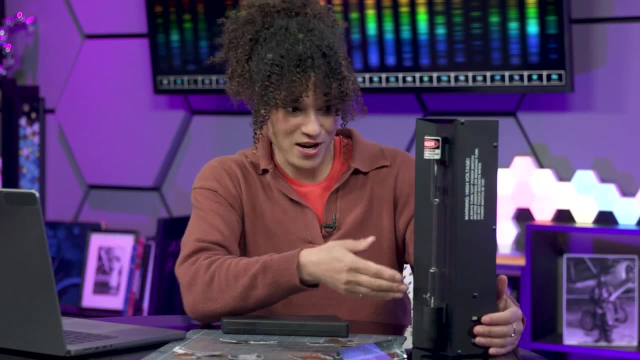 So we have to do experiments on Earth like this to prove what we're looking at, looks like what we are thinking we're looking at. So in here This is argon, and if we turn it on here, it glows as really pretty purple. 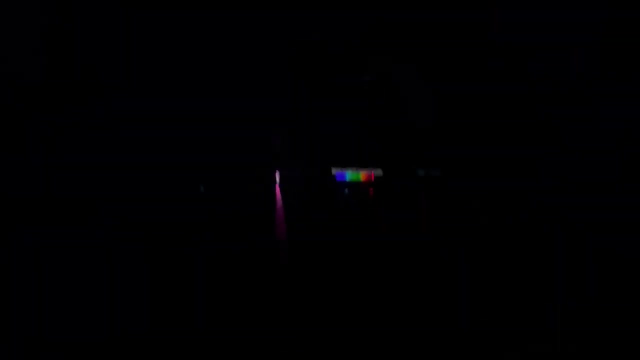 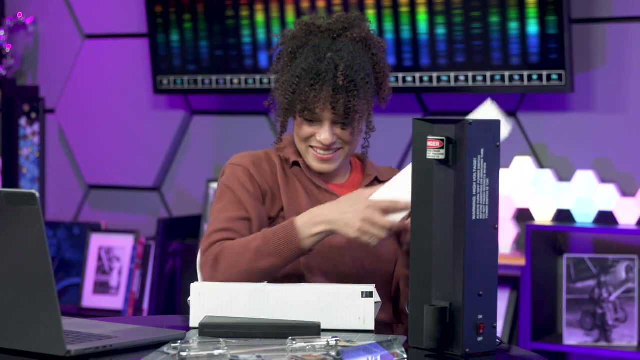 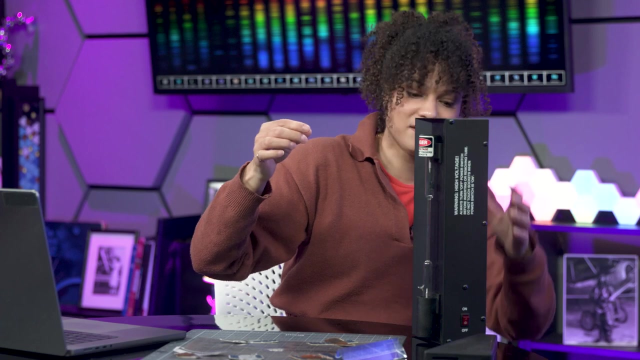 And then, if we look at it with a spectroscope, it shows us a very specific fingerprint to argon. These are called spectral tubes, My bounty of tubes. They contain the gas of one element and the box runs a voltage through the tube. 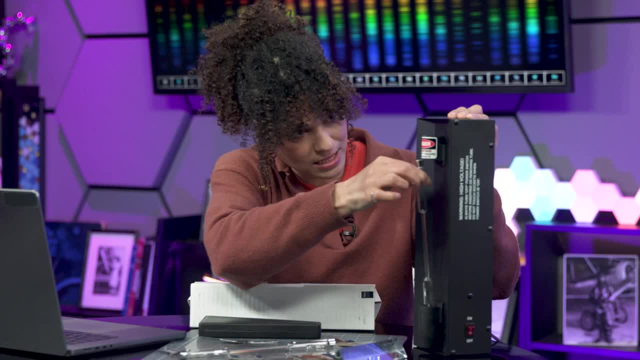 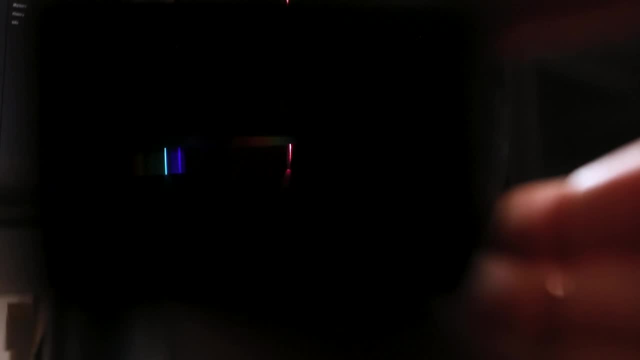 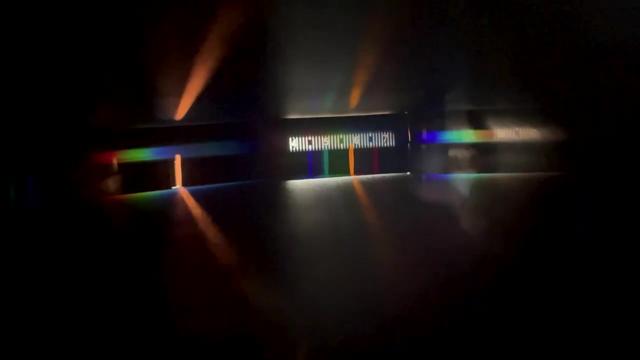 When I turn on the switch, the charged gas turns to plasma. Amazing. It emits a color that is unique to that one element. It also makes unique lines when you look through the spectroscope. This one is helium. This same process happens in a star or a hot region of gas. 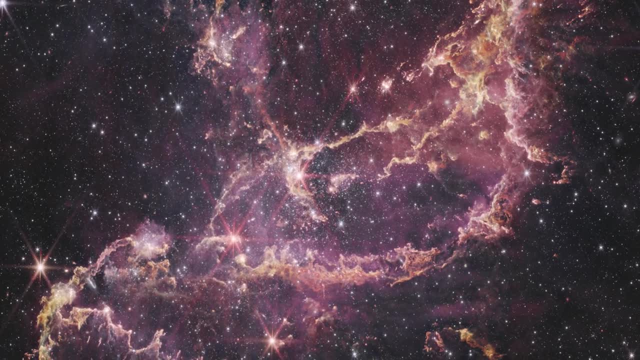 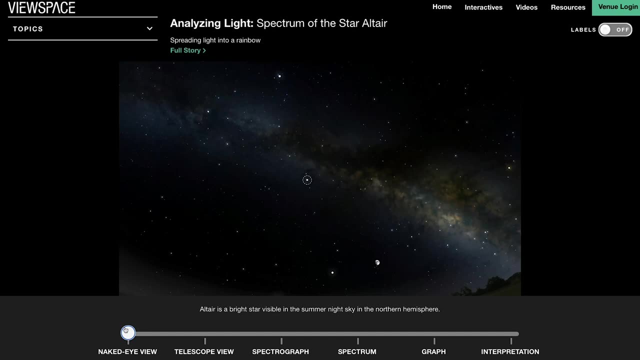 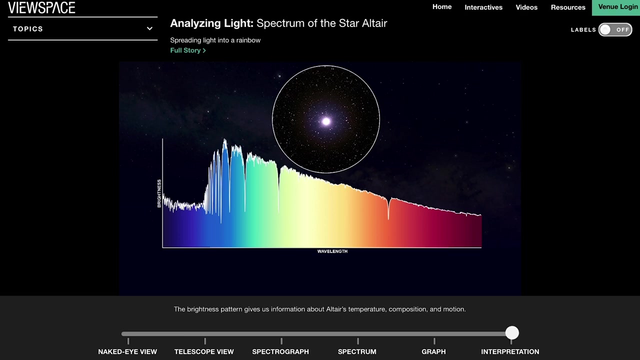 So we use tubes like this to verify what we see in space. If you do a quick search for spectroscopy data, there are numerous ways that the data can appear. Those variations are based on the source of the cosmic light. There are three types of spectra that we can use. 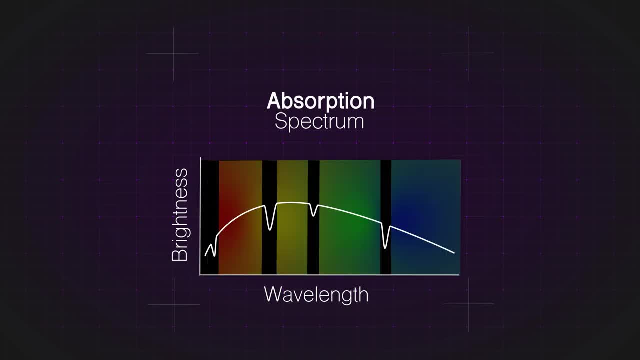 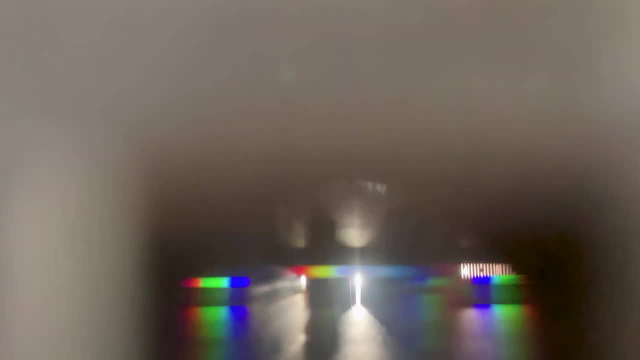 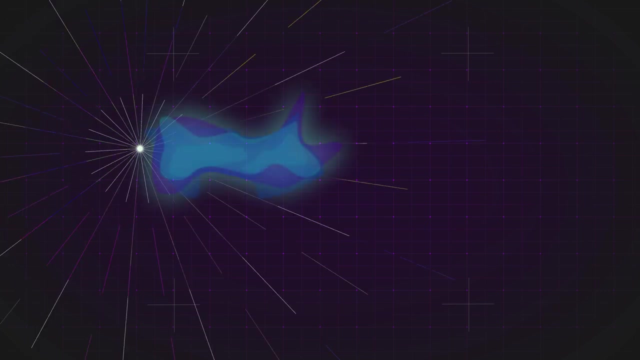 Continuous emission and absorption. Light from a hot, dense source like the sun produces a continuous spectrum. When that light passes through cooler gases on its way to us, the gases take away or absorb some of that energy. Dark lines appear. 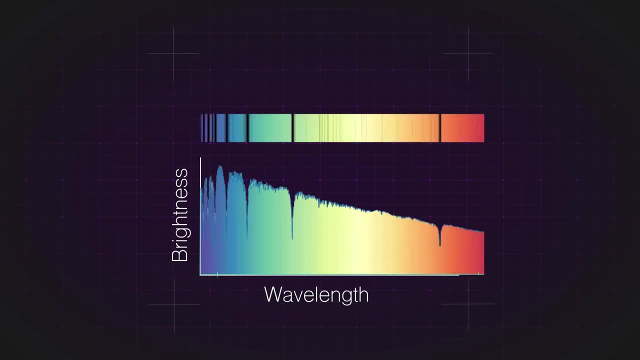 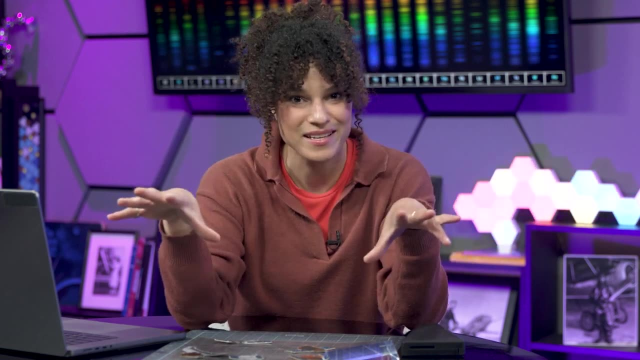 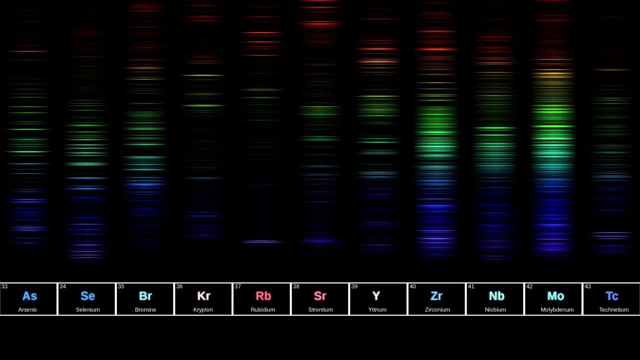 Where, Where specific colors are missing And when thin gases glow themselves, we see only their characteristic colors, kind of like a cosmic barcode. These are the emission spectra from pure elements that were given a voltage to glow, just like my spectra tube. 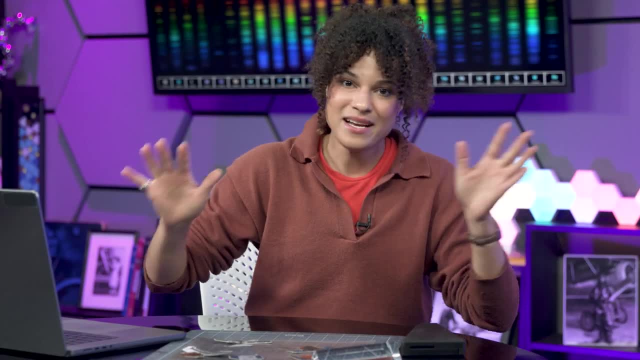 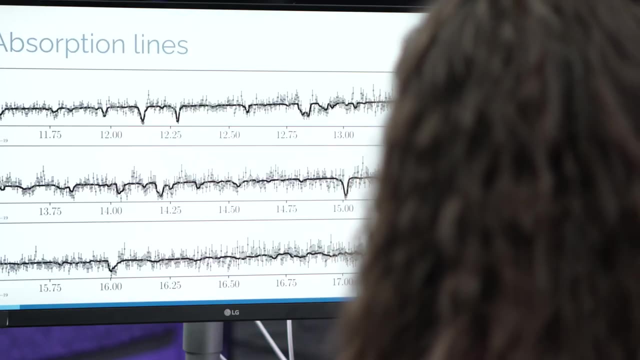 But way better. Like all data, there is an art to analyzing spectra. Scientists like Dr Oozawak use computers to analyze spectra. They use computers to calculate and tease out clear signals, comparing them then to models that are already known. 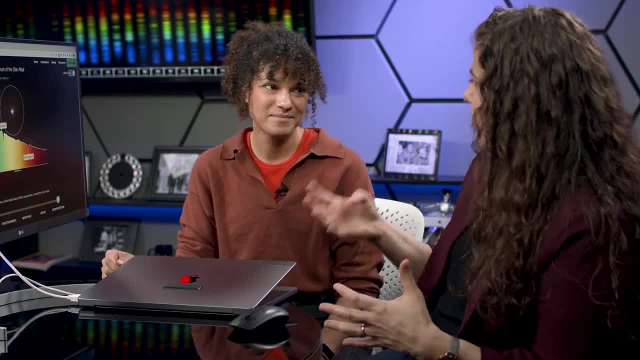 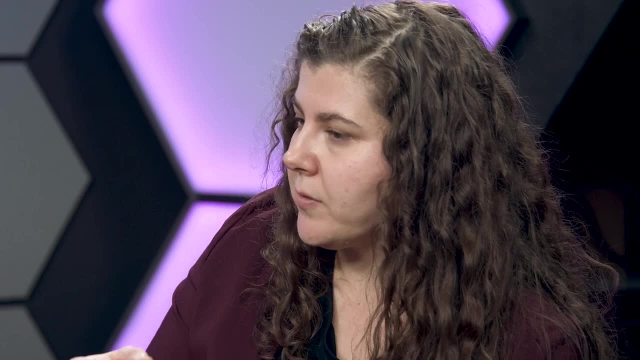 Many scientists in the labs on Earth. they try to recreate the same conditions and measure basically what these kind of, as you said, fingerprints of those different transitions for different elements are Okay. so we're always comparing to sort of the fingerprint of what we have. 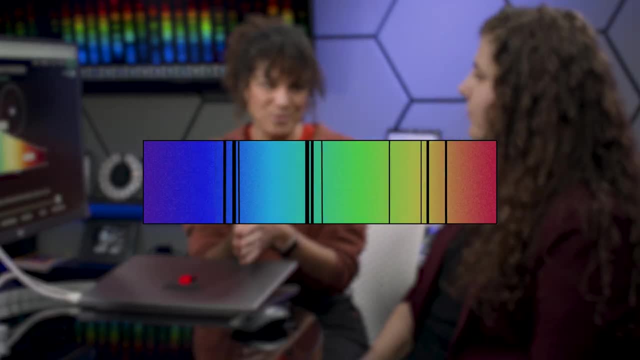 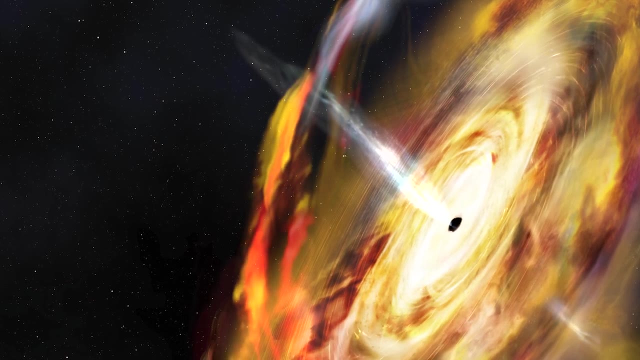 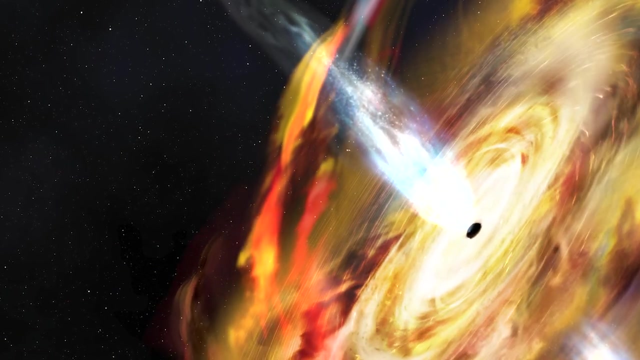 Yes, And then if it has deviated from that, that is the new information from what we're looking at, Correct For Anna. spectra unveil the structures of black holes, the swirling winds that surround them and those big jets of particles that come out of them. 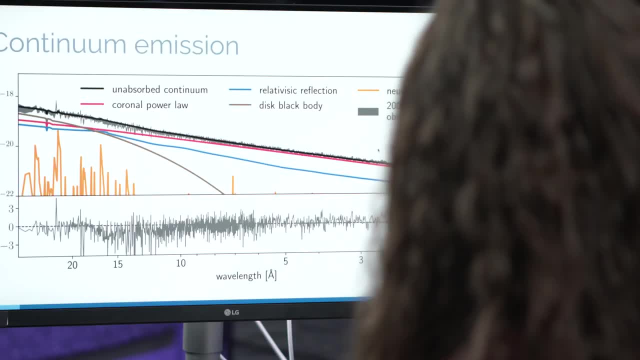 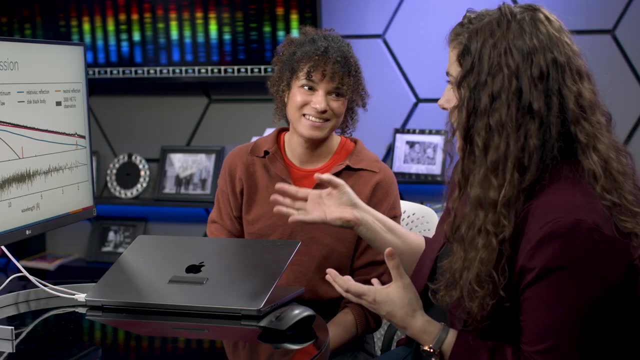 When you look at a black hole, this is what you see. Yes, Where is the accretion disk? Where are the winds? So all of this is mostly accretion disk at this level. It's just different parts of it. 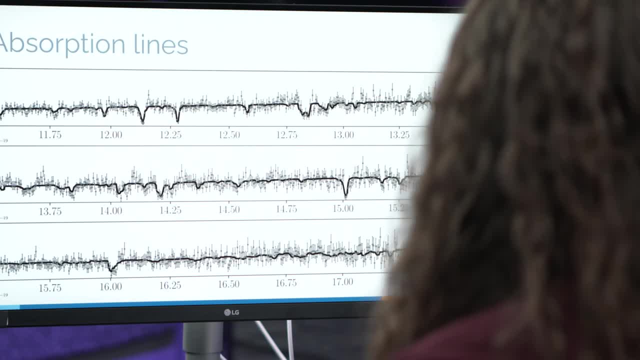 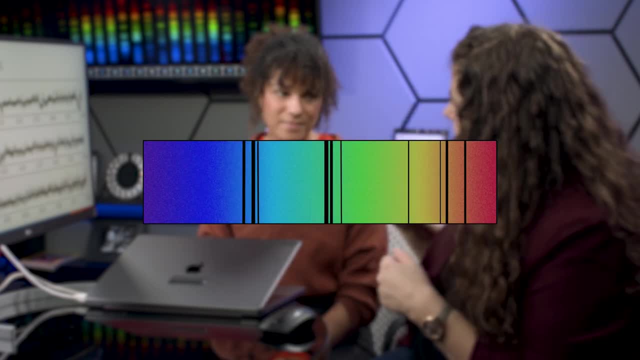 We can zoom in right, Yes, And we see all of the absorption lines right. All of these lines are also shifted a lot, So they come from this wind that we saw in the first picture. So that's how we know that there is wind blowing around black holes.